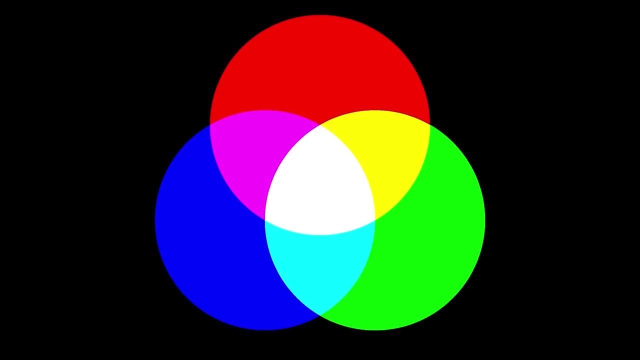 all use additive color mixing. If you were to combine all the primary colors, you would end up with white. However, this is only true if you're using light to mix color. If you were to take the primary colors and mix different combinations together, you'd create colors. 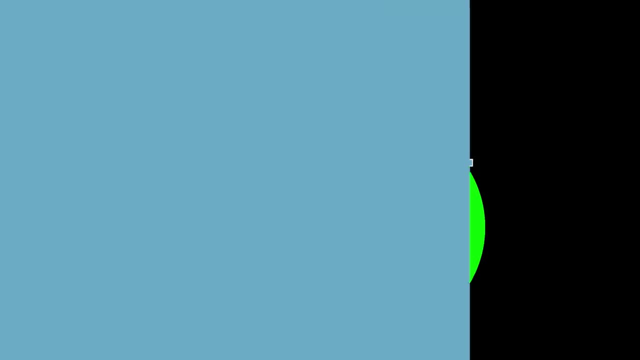 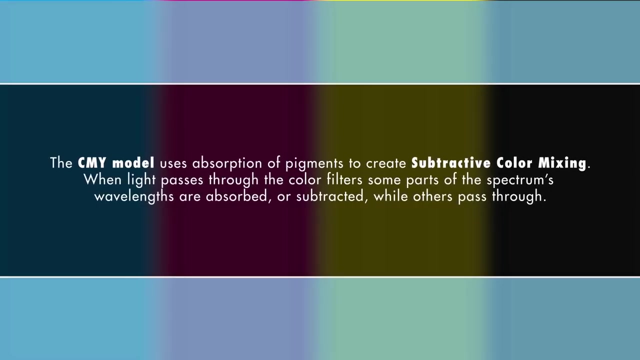 of cyan, magenta and yellow, known as secondary colors. The CMY model uses absorption of pigments to create subtractive color mixing. When light passes through the color filter, some parts of the spectrum's wavelengths are absorbed. Subtractive color mixing can be found in magazines, advertisements and other printed. 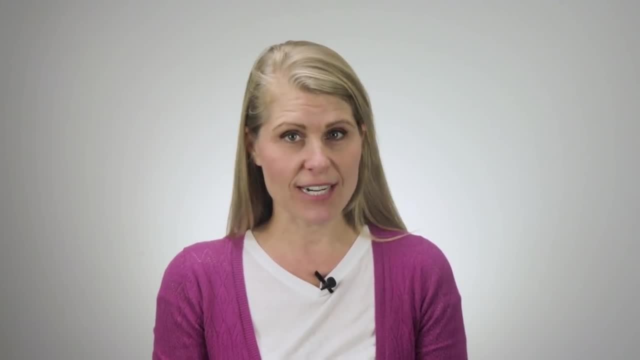 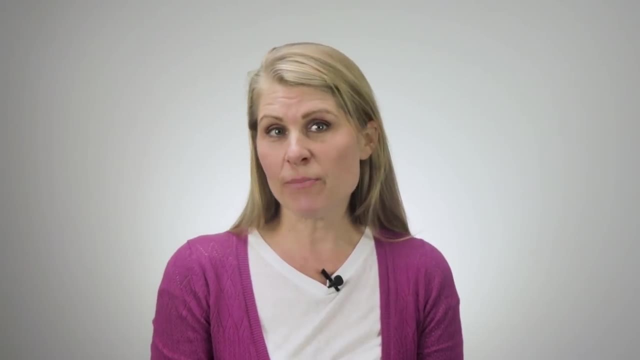 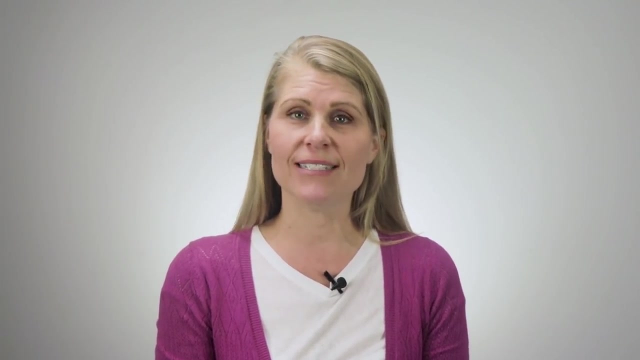 material, And just as additive colors can create subtractive colors, the reverse can be done: Mixing subtractive colors can create primary colors. Now that we've learned a bit about color mixing, it's time to play a game. We talked earlier about how it's possible to create primary colors from secondary colors, so that's going. 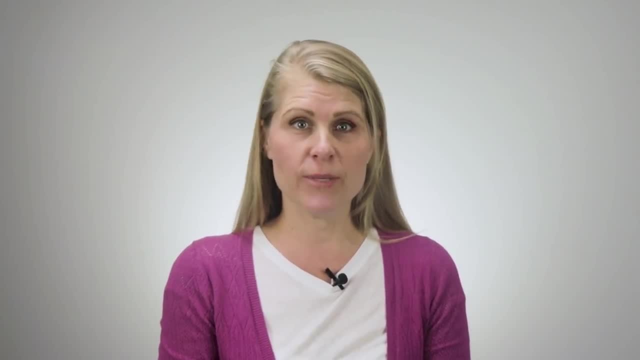 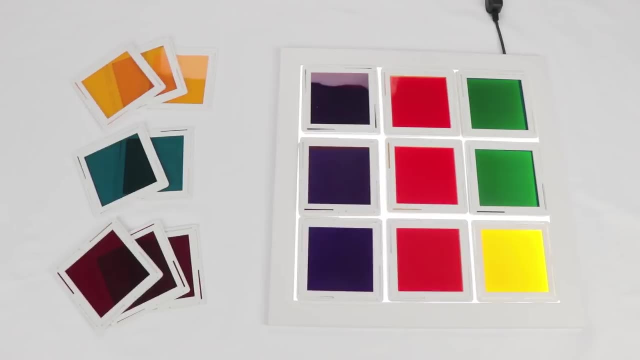 to be our first experiment. Start with one column each of magenta, cyan and yellow, Now using only three yellow, two cyan and three magenta filters. place them on top so that there are three blue, three green and two red, leaving only one space yellow. 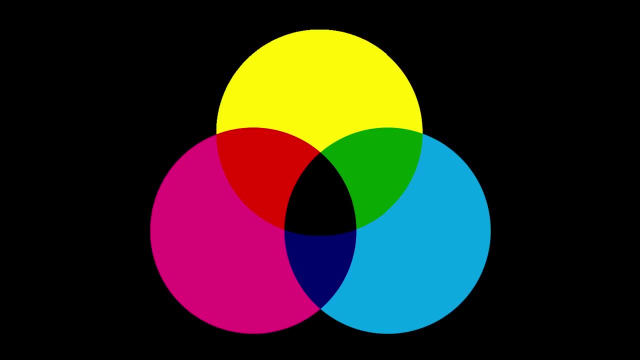 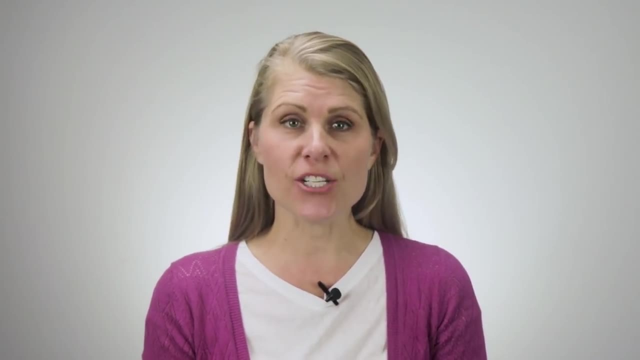 Let's start with the magenta column first. If we take a look at the color wheel and we locate magenta, we'll see that across from that is green. When colors are across from each other, it's an easy way to remember which color is absorbed. So magenta absorbs green. 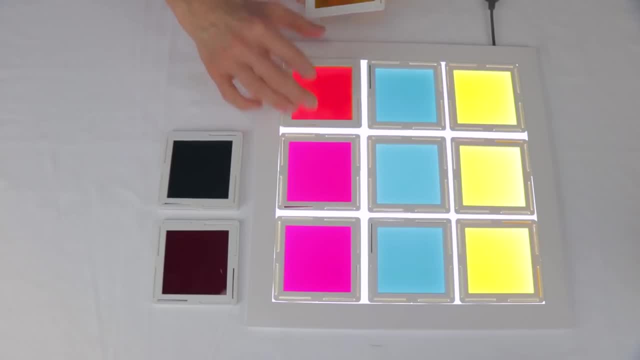 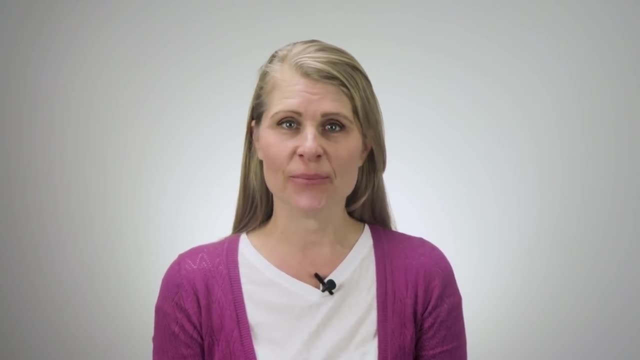 red and blue to show through. In this case we would need to place a yellow filter on top, because yellow is absorbing the blue, which we can confirm by looking at the color wheel again. So when the yellow is added, only red light is visible. 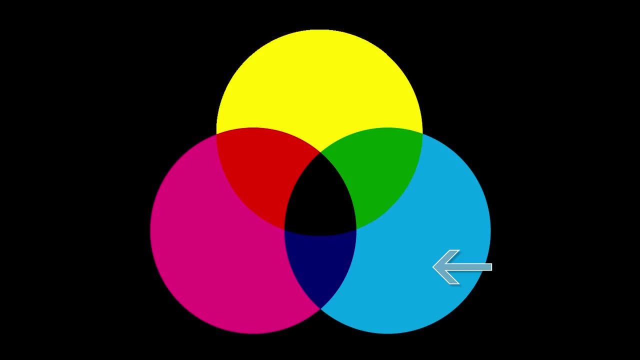 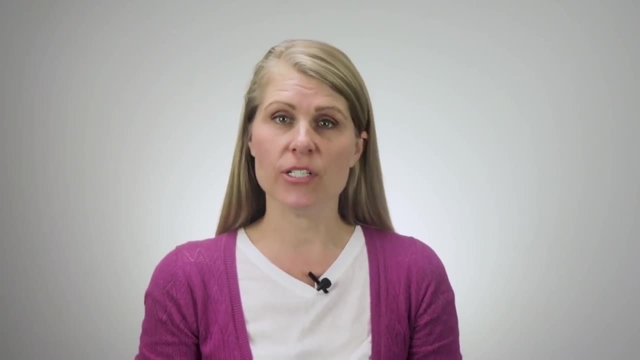 Let's move on to the cyan column. The cyan filter is absorbing red color and allowing green and blue to pass through, So we would need to place a magenta on top, because we now know that magenta allows red and blue to pass through. 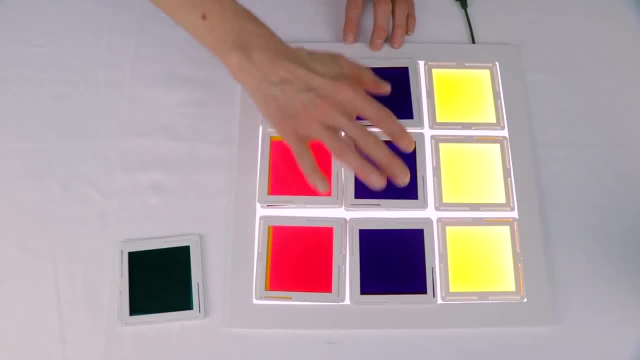 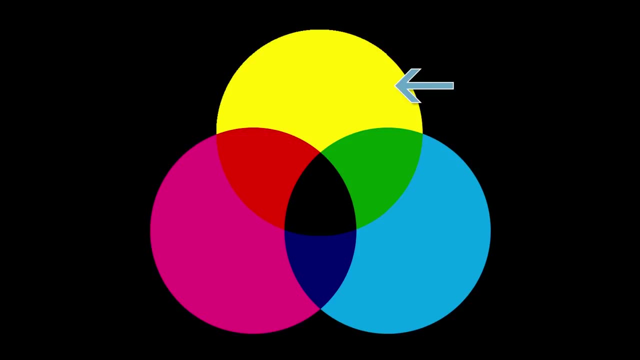 And when placed on top, it's green and blue. Now for the last two yellow filters. we already know that cyan allows green and blue to pass through, But yellow filters absorb blue and allow red and green to pass through. So when 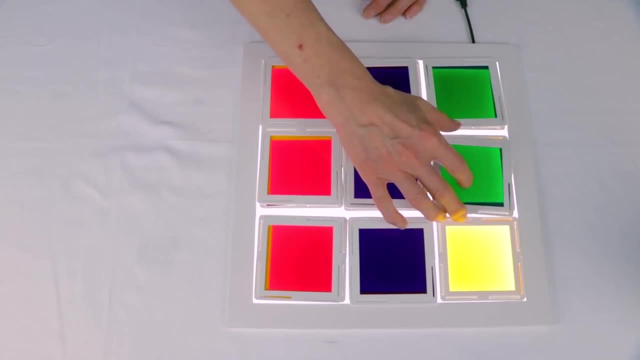 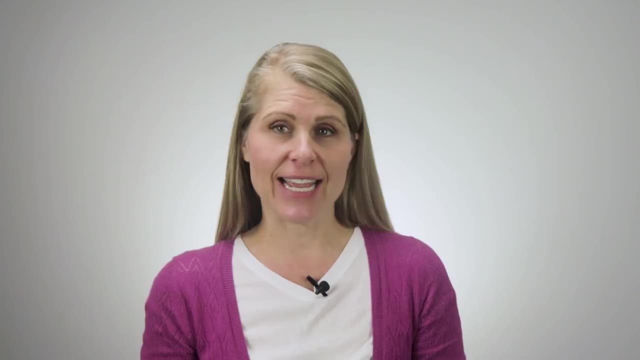 we place the cyan on top, the color becomes green. And for the final yellow we'll just leave it as it is. Let's try another one. Start with magenta, cyan and yellow. like in the first experiment, Using three green, three red and two blue filters arrange the 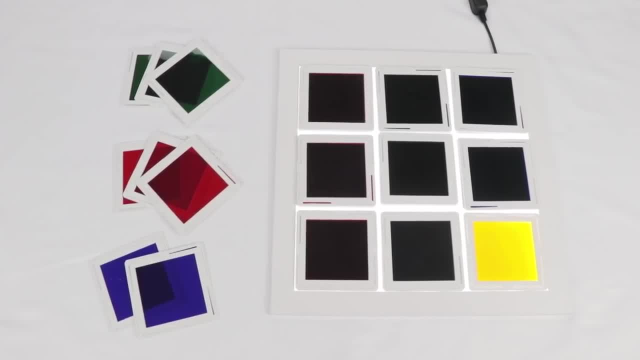 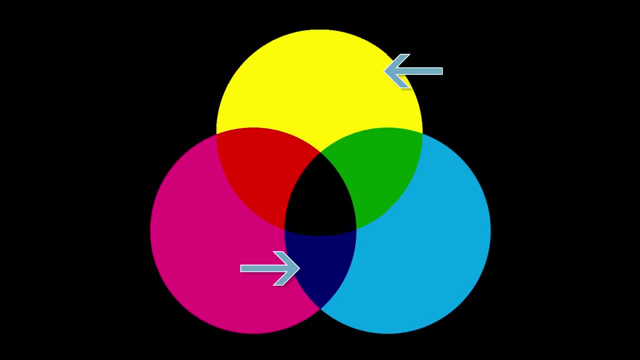 board to produce a nearly completely blacked out pattern like this. Let's start with the yellow filters first. From everything we've learned so far, we know that yellow filters absorb blue. So if we were to use the blue filter, our result should: 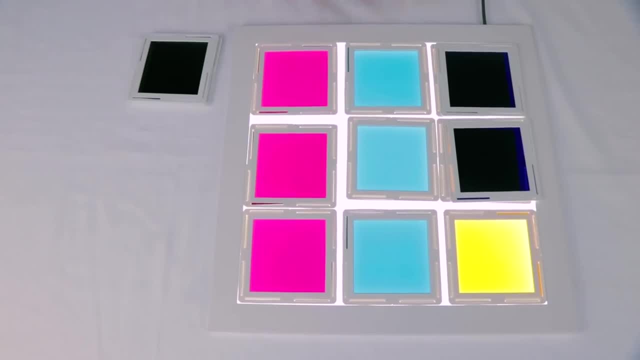 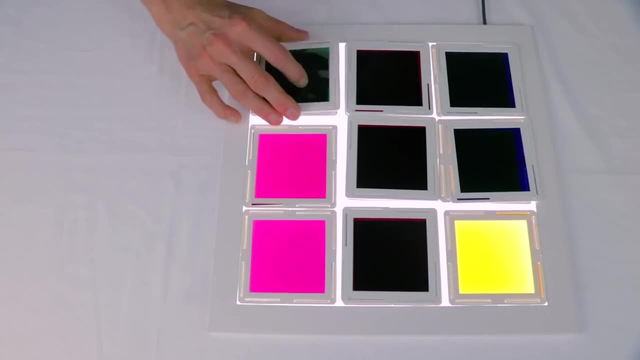 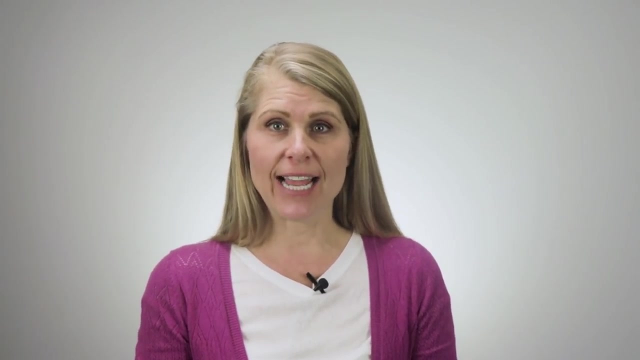 be black For the cyan? we know that it absorbs red, which gives us our black. And finally, the magenta absorbs green. And what do you know? that's the last filter we have Today. we've learned a little about subtractive and additive color mixing using a few puzzles. 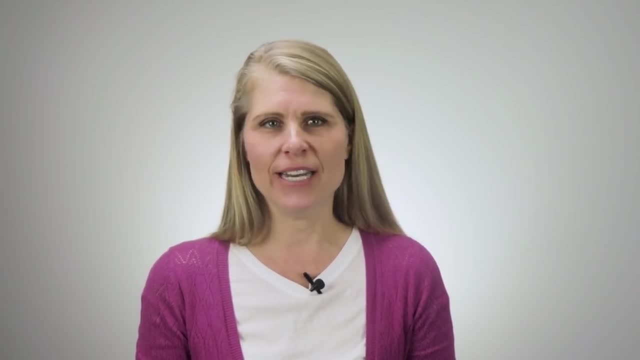 But what's also cool about this device is you can create your own color combinations or experiments. 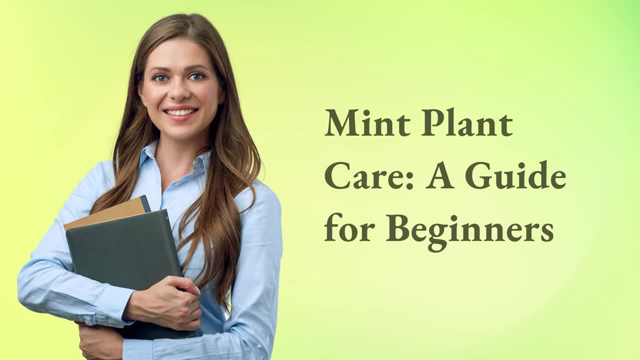 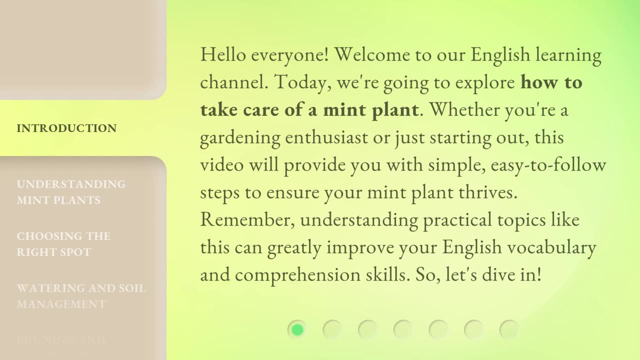 Mint Plant Care – A Guide for Beginners. Hello everyone, welcome to our English learning channel. Today we're going to explore how to take care of a mint plant. Whether you're a gardening enthusiast or just starting out, this video will provide you with. 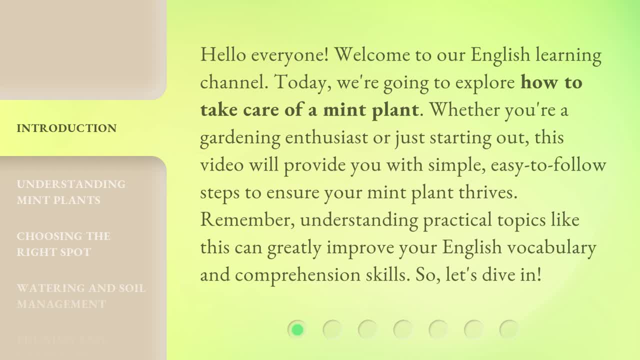 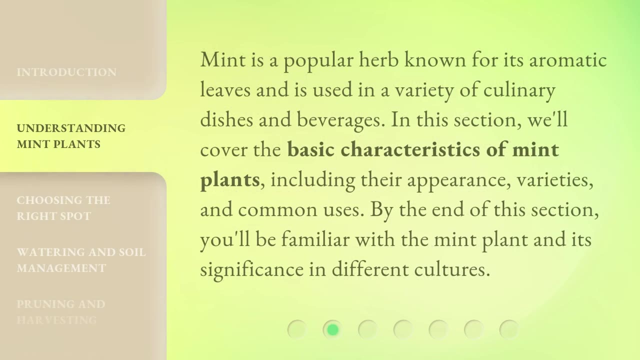 simple, easy-to-follow steps to ensure your mint plant thrives. Remember: understanding practical topics like this can greatly improve your English vocabulary and comprehension skills. So let's dive in. Mint is a popular herb known for its aromatic leaves and is used in a variety of culinary. 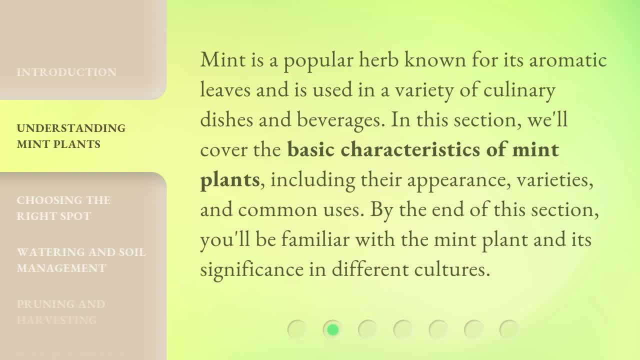 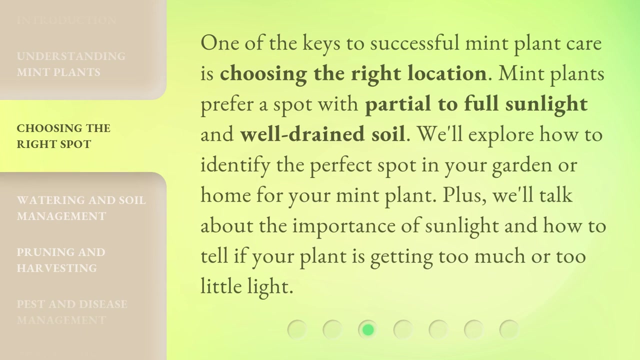 dishes and beverages. In this section we'll cover the basic characteristics of mint plants, including their appearance, varieties and common uses. By the end of this section, you'll be familiar with the mint plant and its significance in different cultures. One of the keys to successful mint plant care is choosing the right location.